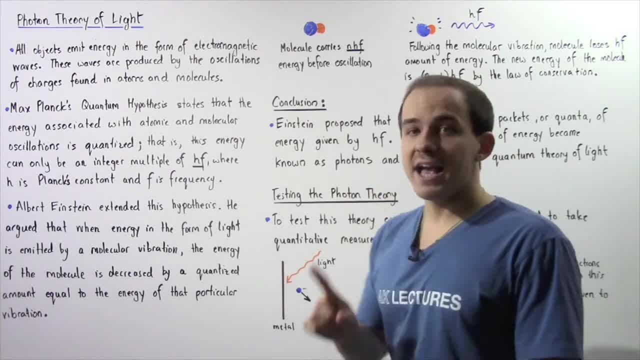 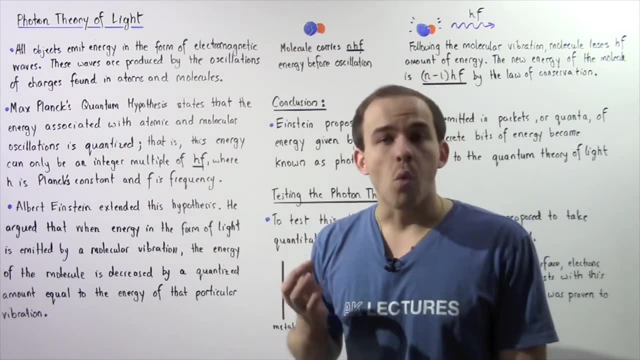 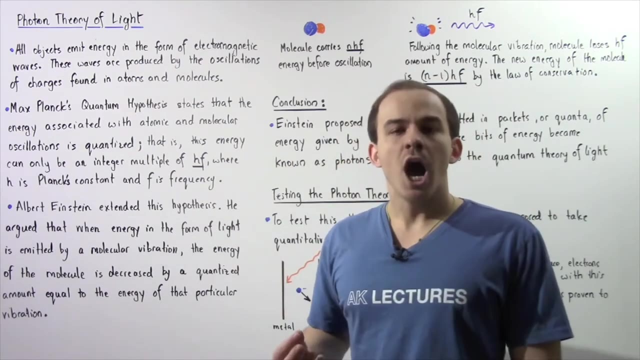 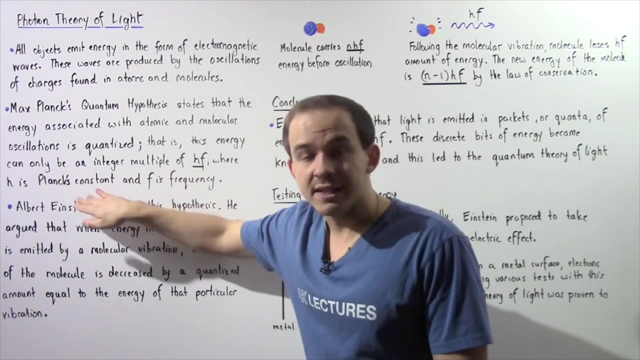 we spoke about in the previous lecture states that the energy associated with atomic and molecular oscillations is quantized, That is, this energy can only exist as an integer multiple of the minimum energy given by h times f, Where h is Planck's constant- it's a value that was calculated experimentally- and f 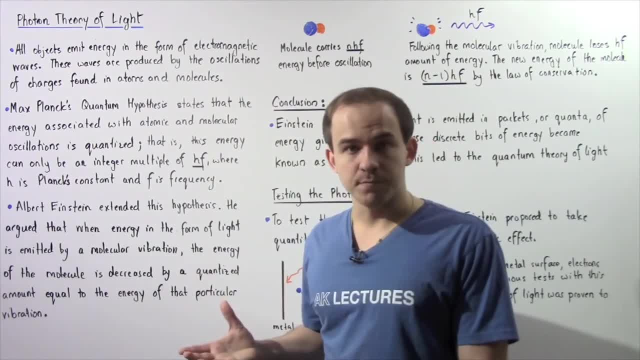 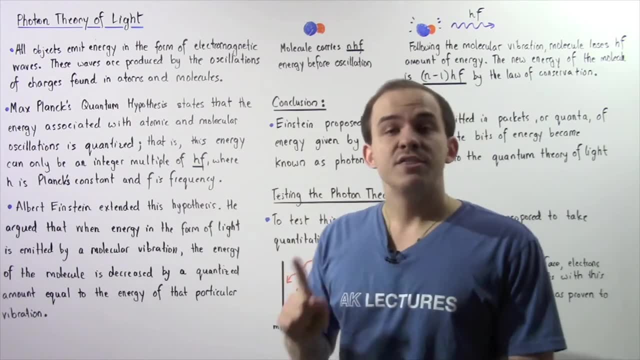 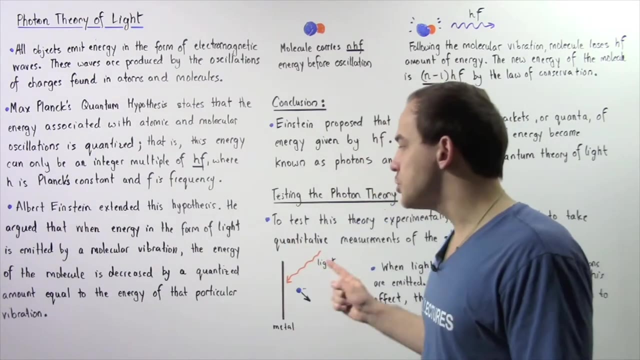 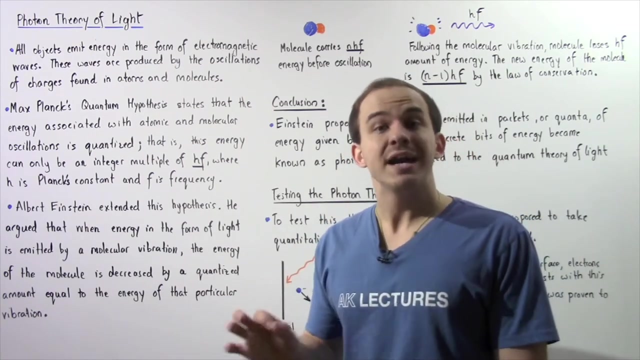 is the frequency of that particular oscillation. Now Einstein extended this hypothesis even further. He argued that whenever energy is emitted in the form of light by a molecular vibration, the energy of that molecule is decreased by a constant. This is the reason why, upon calculation, we know that some people do not know that a 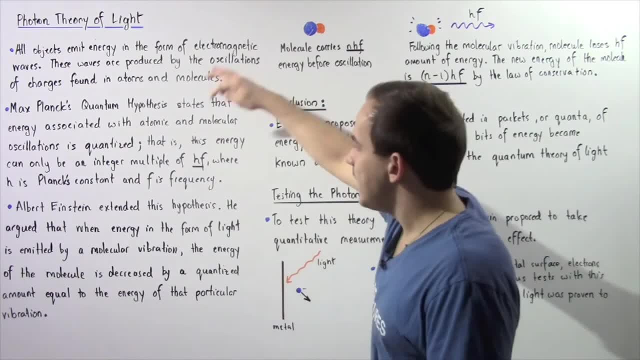 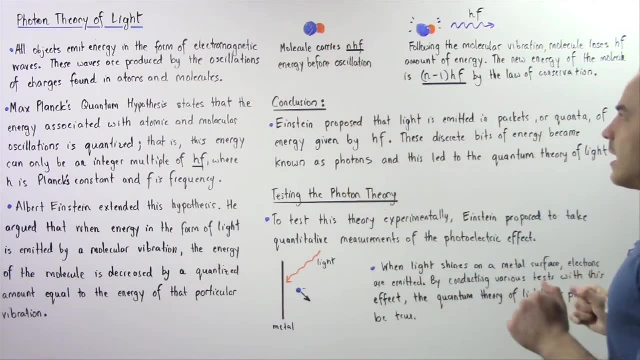 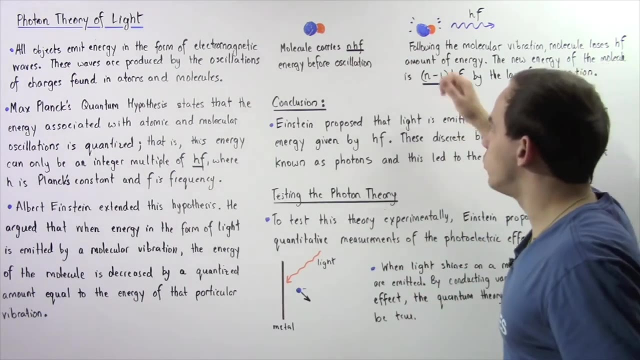 force, of force is guaranteed and they do not know that a power is going to be generated at that particular moment. earlier, let's look at a shape, that of vinegar sugar, liberal sugar, that we can consider a sizable composition immediately after class to Trine and Ich, as anything but a mass pressure. 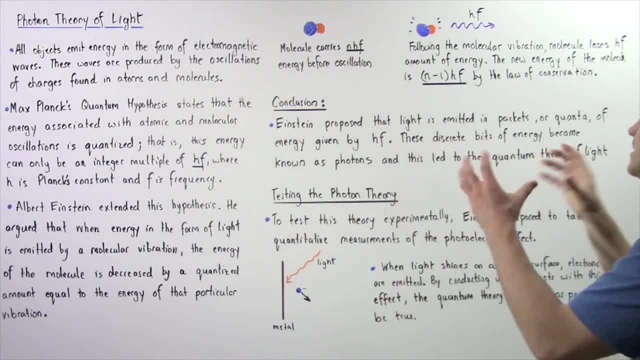 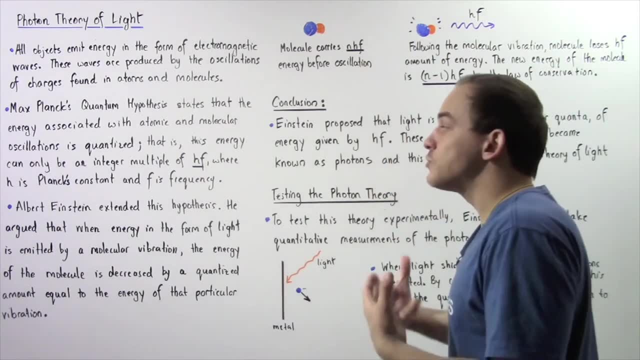 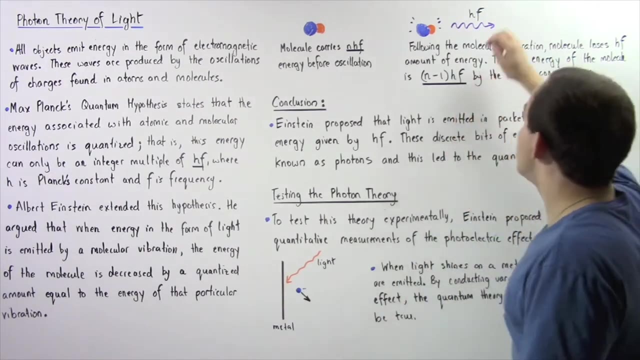 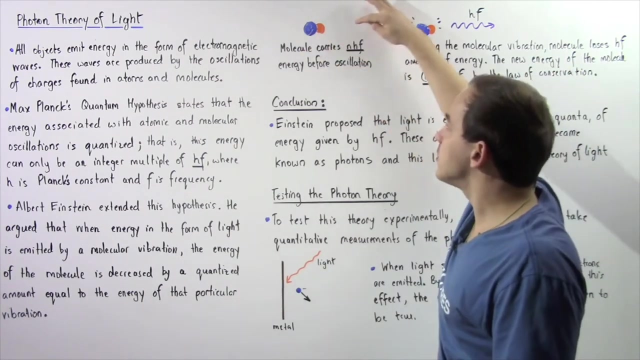 a duration that value? Now, once our oscillation, once the vibration of the molecule actually takes place, it emits electromagnetic wave in the form of light. That light carries an energy that is quantized, that is equal to H multiplied by F. Now, if the initial energy of our molecule was N, 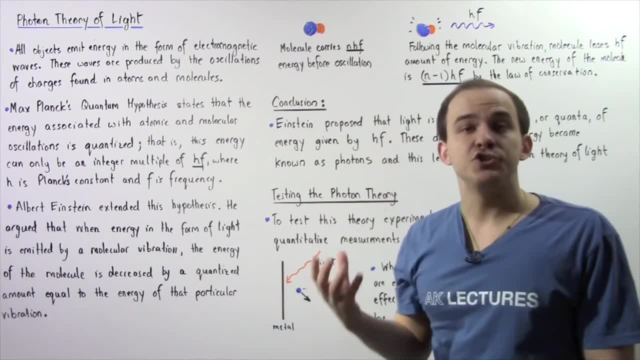 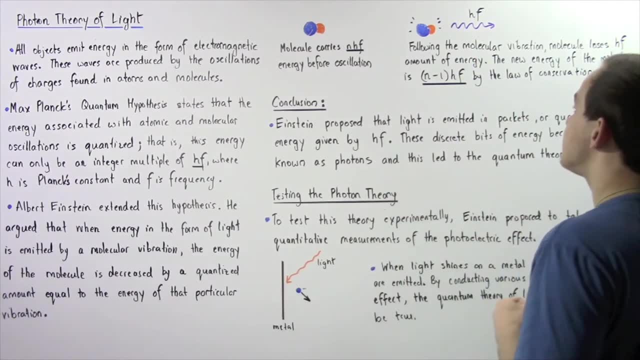 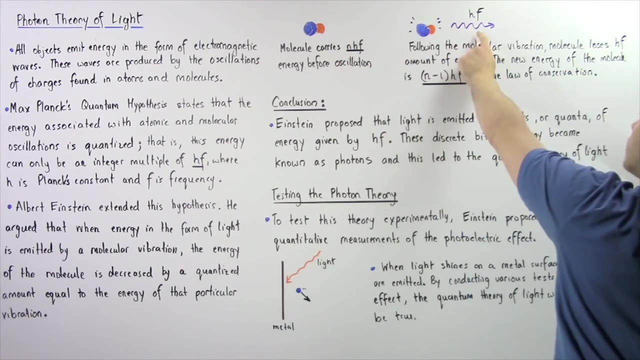 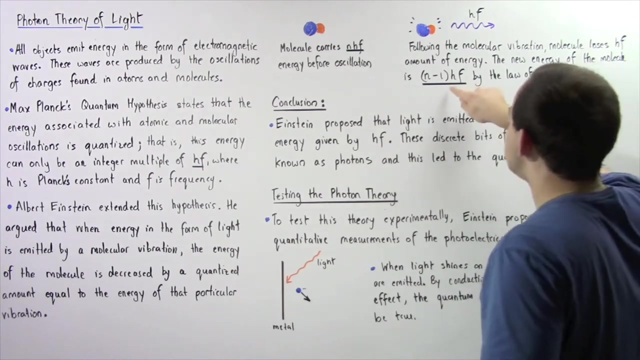 times H times F, and because energy is conserved, that means the final energy of the system of the molecule after that oscillation is equal to N times H times F, minus the energy it lost in the form of emitted light, H times F, and that is equal to N minus 1 times H times F. So by making